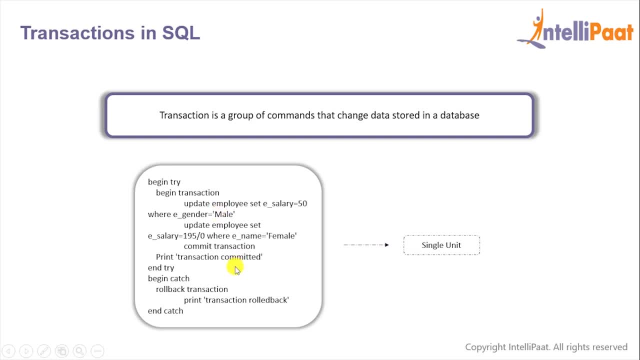 that either all of these commands are executed successfully or none of them is So. let's say, if one of the commands in the transaction fails, then all the commands will fail and any data which was modified in the database will be rolled back. Similarly, if all the commands inside the 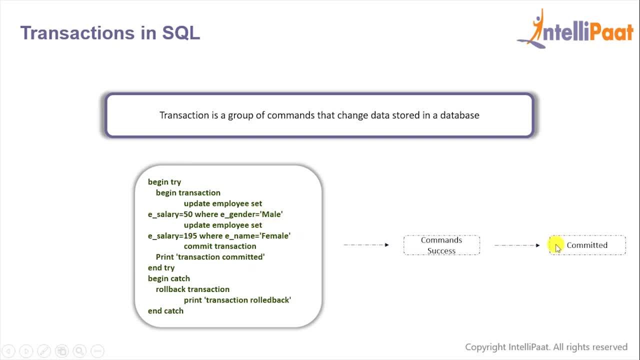 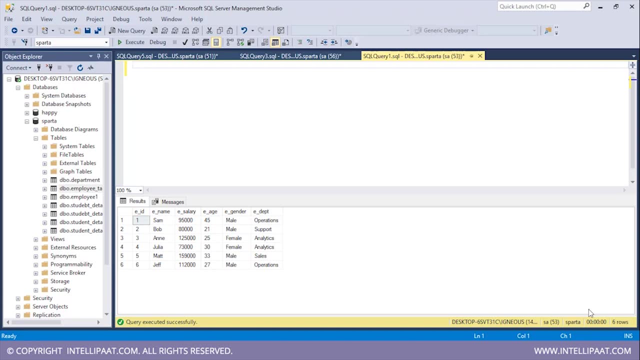 transaction execute successfully. only then the transaction will be committed. So this is how transactions ensure integrity of data. So now I'll begin a transaction and inside that transaction I'll try to update this age value from 45 to 30.. So let me write the syntax. 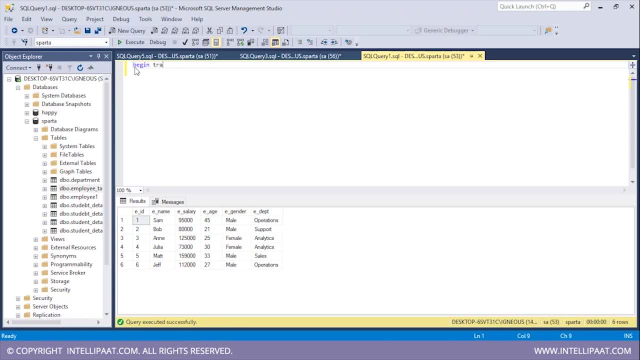 To begin a transaction. So I'll type begin and then type transaction And inside this I'll give all of those SQL statements which either have to be committed or rolled back. So over here I'll give the update statement, I'll type update and then give the name of the table which would 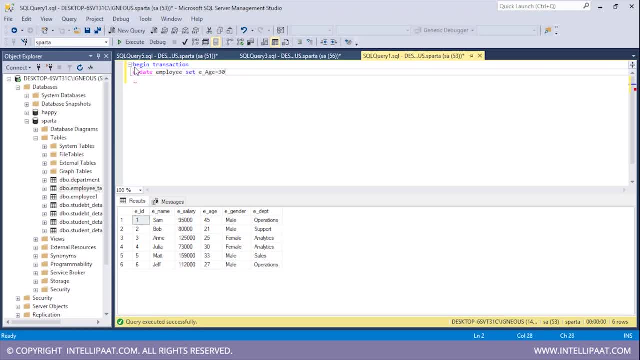 be employee. Set e age to be equal to 30 where e name is equal to Sam. So I'll select these two statements and I'll execute them. So we see that one row has been affected. So now let me have a glance at the modified table. So I'll type: select star from employee. I will select this. 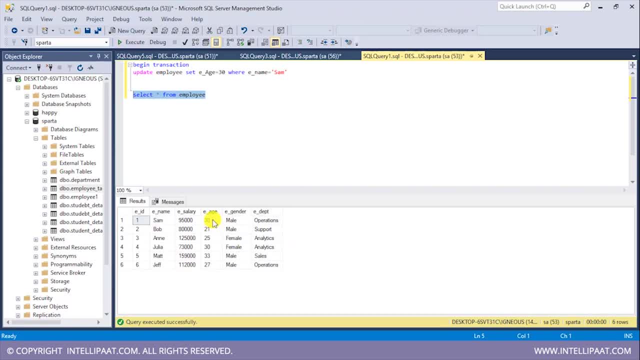 command over here. I'll execute this right. so see that initially the age value was 45. And after we apply this update command, the age has been changed from 45 to 30.. Now, since this command is inside a transaction B, have the. 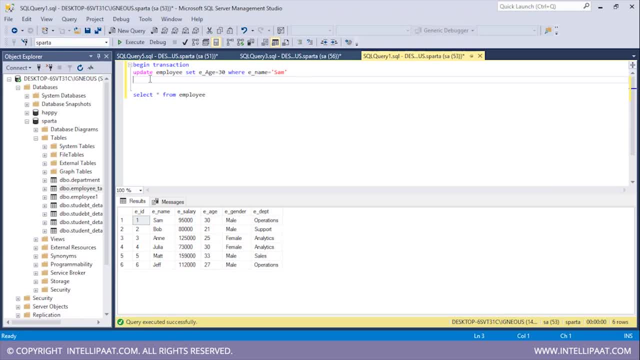 lu this command or commit this command. So now let me go ahead and actually roll back this transaction. So to do that, I'll type rollback transaction. So now let me select this. I'll click on execute So we see that the commands have. 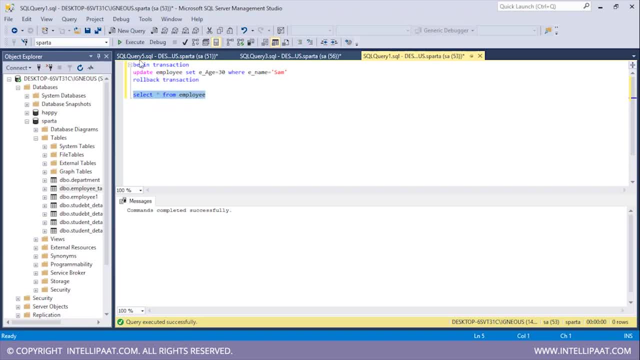 been completed successfully. Now let me again have a glance at the employee table Right. so since we have rolled back the transaction, we see that the age value has gone back to the original value, which is 45. So initially, using the update command, we had changed the age value from 45 to 30, and after that we 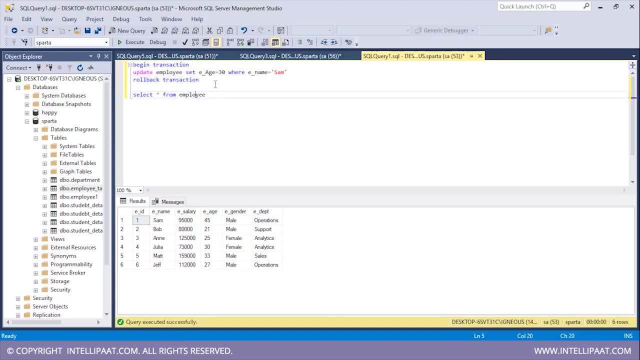 had rolled back the transaction. Now, what I'll do is I'll execute these two statements again and let me have a glance at the table Right. so again we see that the age has been changed to 30. So this time, instead of rolling back the 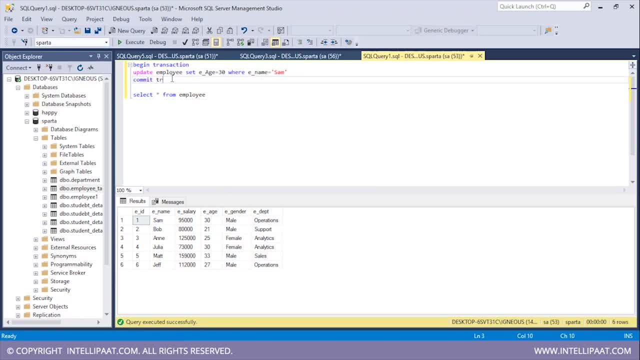 transaction. I will commit the transaction. So I'll type commit transaction. So I'll type commit transaction, So I'll select this, I'll click execute. Now let me have a glance at the table. So this time the transaction has been committed and the change is. 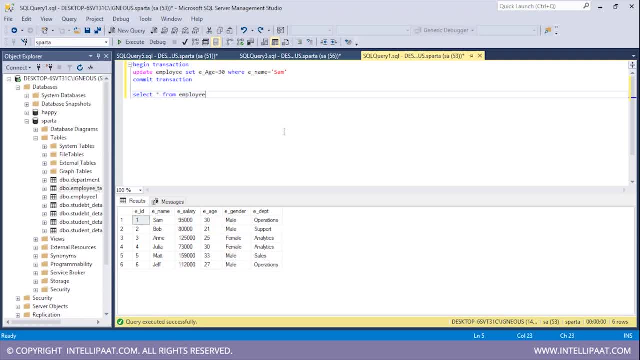 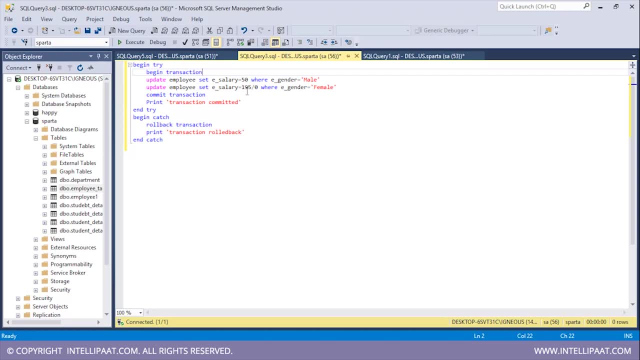 permanent. So this is how we can either commit or roll back the commands using the transaction. Now let's look at another example. So in this example we are using transactions inside the try-catch block. So over here we are beginning the try block and inside this we are beginning the transaction, And inside 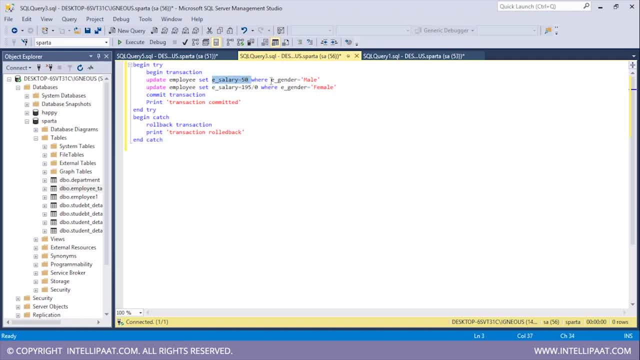 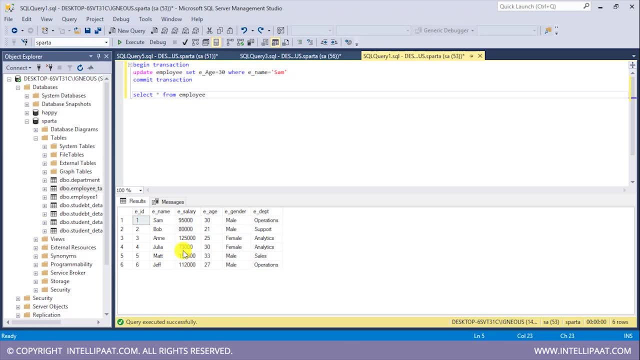 the transaction, we are trying to update the salary value to be equal to 50 where the gender value is equal to male. So wherever the gender is equal to male, we'll update that salary value to be equal to 50.. Similarly, wherever the gender value 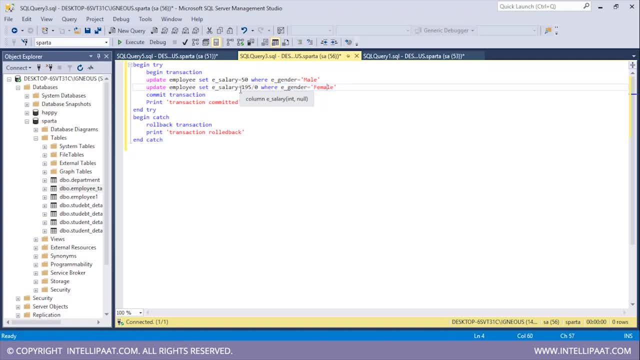 is equal to female, I will change that salary value to be 195 divided by 0, which would give us an undefined value, And after that we'll commit this transaction and print transaction committed Now, since we have put this transaction inside the try block, if any. 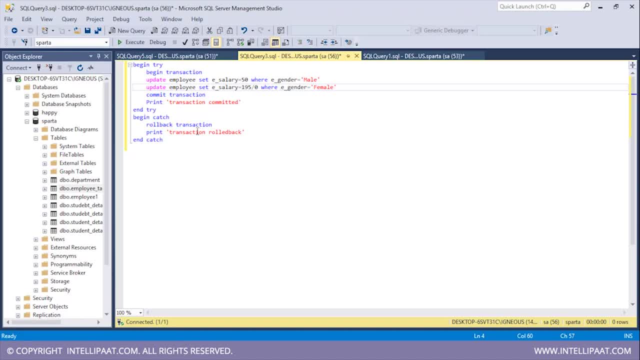 error occurs, that will be sent to the catch block and we will roll back the transaction. So over here we see that we are dividing 195 with 0. And since this gives us an undefined value, we will get an error And that error will be handled. 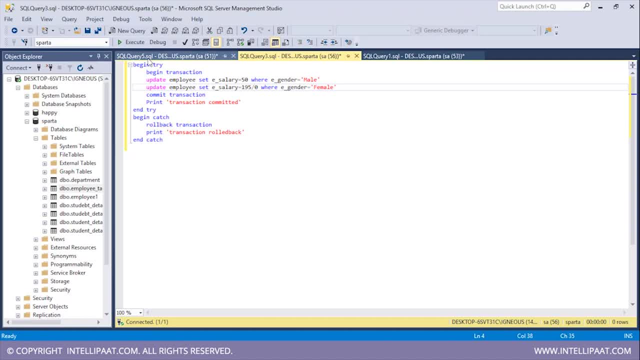 in this catch block and we will roll back the transaction. So let me execute this. So you see that the transaction has been rolled back Because we get an error inside the try block. Now what I'll do is I will remove this divided by 0 and run this command again. So this time we see that the 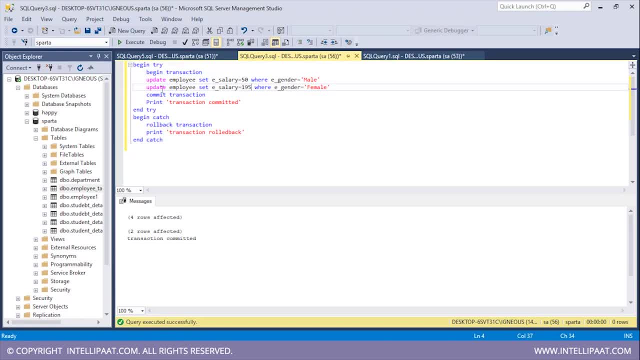 transaction has been committed because there was no error inside the try block. So now let me have a glance at the modified employee table. So I'll type select start from employee, I'll select this, I'll click on execute Right, So we